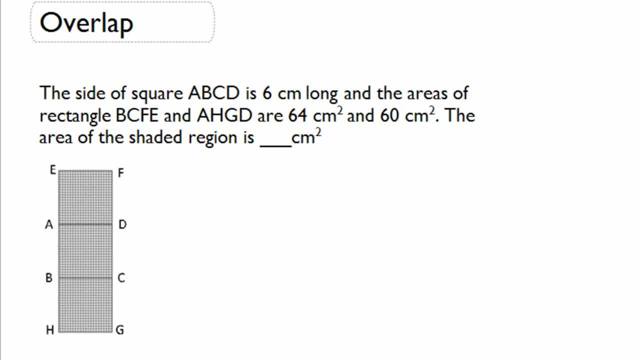 Now let's talk about how to solve problems that involve overlap. The question says the side of square ABCD is 6 centimeters long. Now, if we know that this is 6 centimeters long and we know that it's a square, we're going to be. 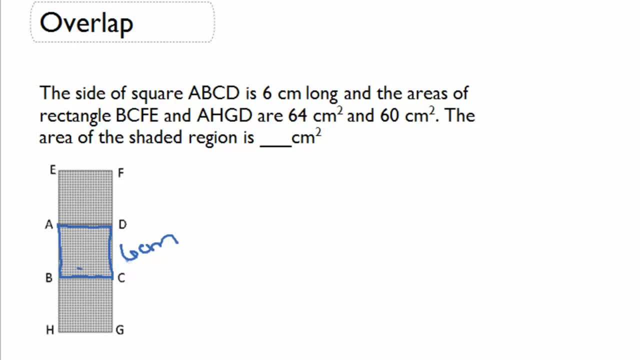 able to find out the area. We're also told in the question that the areas of rectangle B, C, F, E, that total area there is going to be 64 centimeters squared and the area of A, H, G, D, that area is going to be 60 centimeters. 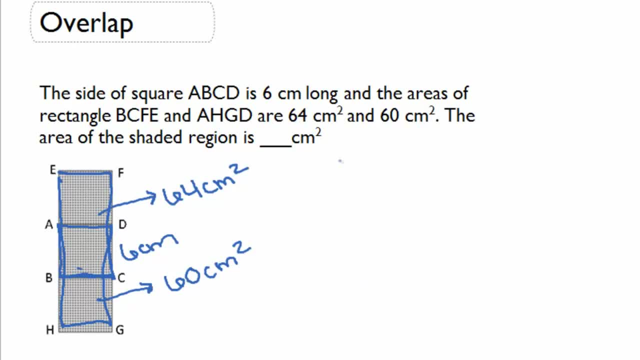 squared. So if we know that we have our two different rectangles, I'm going to redraw this one in green so that we can see the two different rectangles that we have here. We have one on the bottom and one on the top and they overlap and the part. 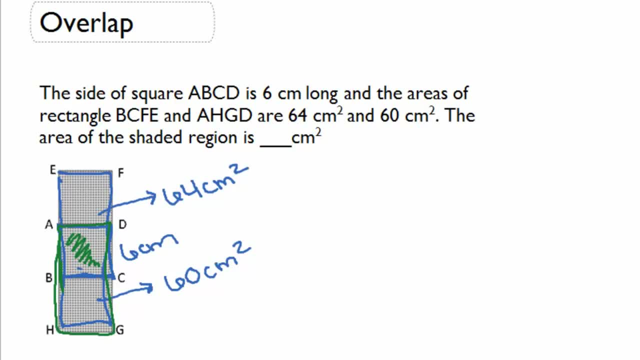 that they overlap in is this part right here, the ABCD square. So if we know that they overlap in that one spot and we figured out the area of that one spot, then we could simply add 64 centimeters squared Plus 60 centimeters squared to find a total of a hundred and twenty-four. 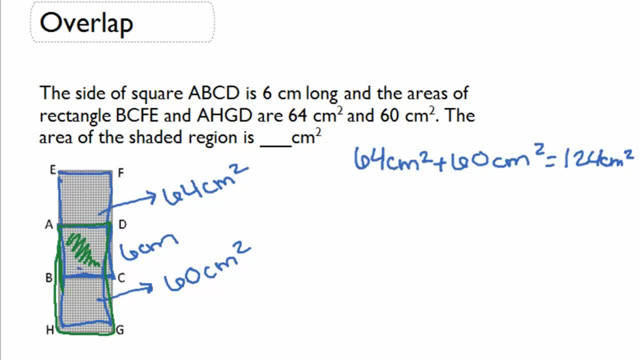 centimeters squared and we could subtract the part that they overlap and we would find the total area. So the area of this part right here is six centimeters squared times. I'm sorry, six centimeters times six centimeters is going to equal equal 36 centimeters squared. and if we subtract that from the 124. 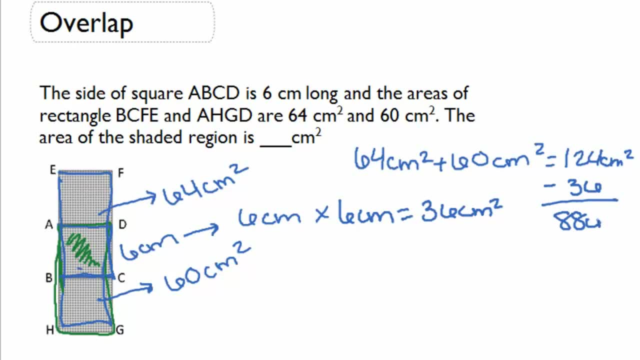 then we're going to get a total of 88 centimeters squared. so if we cut that off because it's overlapping, we would have a total area for our shaded region of 88 centimeters squared.